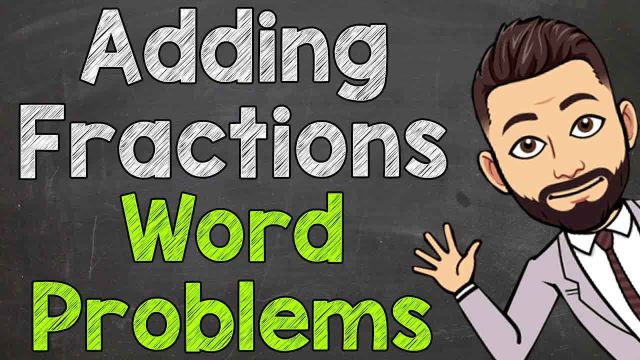 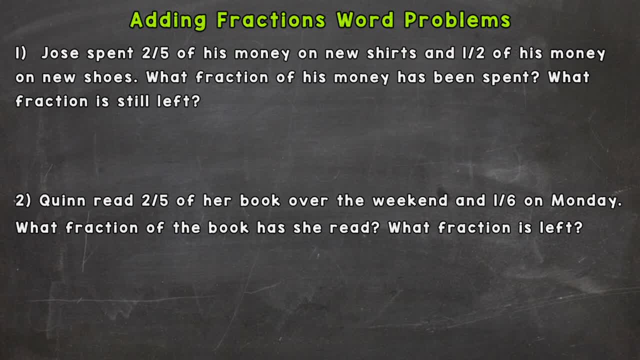 Welcome to Math with Mr J. In this video we're going to take a look at adding, fractions, word problems, and we're going to go through two problems or situations where we'll use adding in order to get us to our answer. So let's jump right into number one here, where we have 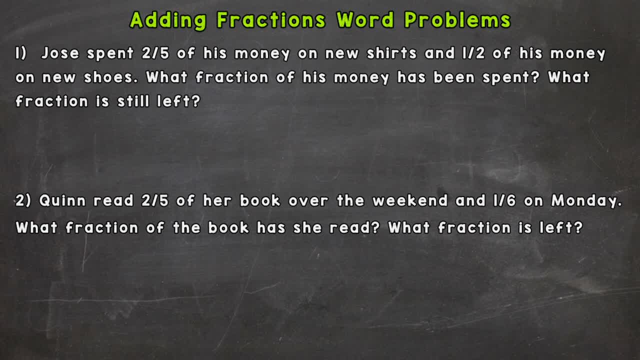 Jose spent two-fifths of his money on new shirts and one-half of his money on new shoes. What fraction of his money has been spent and what fraction is still left? So let's take the information from the problem here. We have two-fifths on shirts and we're combining that. 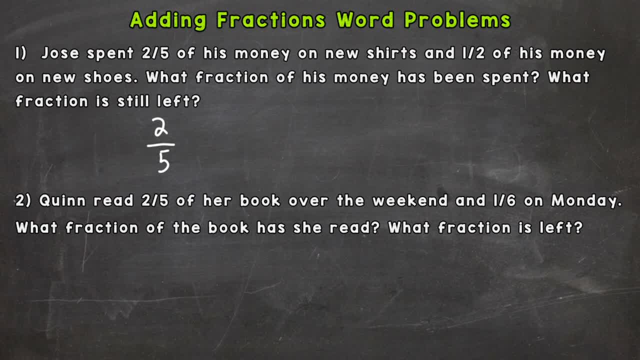 with how much he spent on shoes, which would be adding together. Whenever we have combining of things, it's going to be addition. So two-fifths plus one-half. Now we do not have a common denominator, so we need to find one for five and ten. So the common 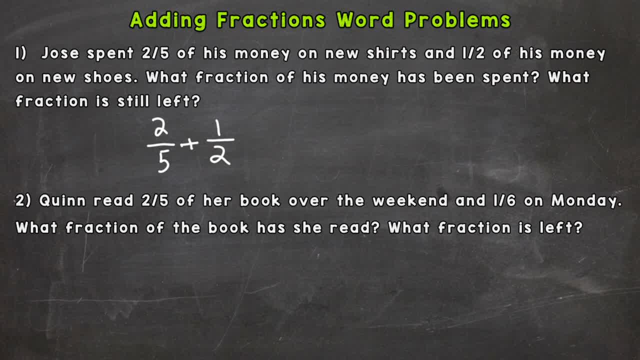 denominator is going to be ten for five and a two. So I'm going to rewrite the problem to the right here. and we have a common denominator of ten. Well, two-fifths, I know, five times two gives me that denominator of ten. so I need to do that to the top in order to get an equivalent fraction. 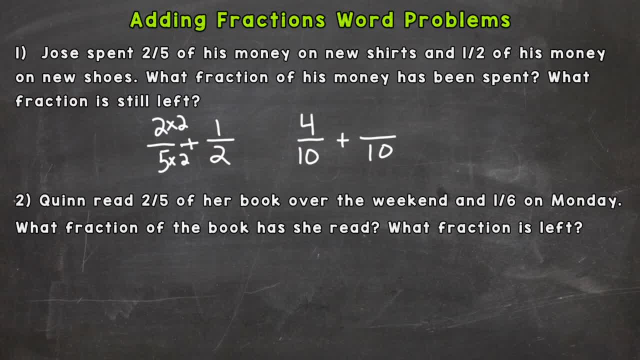 And two times two is four. So two-fifths is four tenths equivalent to four tenths. Now we need to rename one-half. Well, two times five is ten. Let's do that to the top to get our equivalent fraction. One times five is five. Now we're ready to add because we have a common denominator: Four plus five is nine. 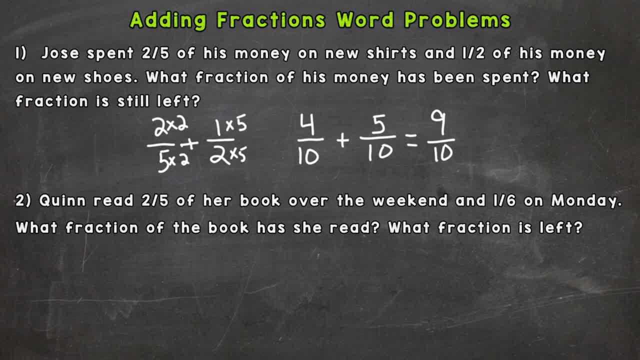 And we keep our denominator of ten the same. So this is how much he spent. He has spent nine-tenths of his money, So nine-tenths has been spent. So now we need to figure out what fraction of his money is left. How do we get to the full? one whole or ten out of ten? So what's left? So if he spent, 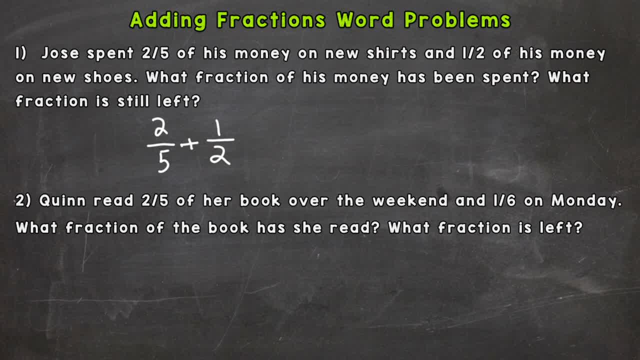 denominator is going to be ten for five and a two. So I'm going to rewrite the problem to the right here. and we have a common denominator of ten. Well, two-fifths, I know, five times two gives me that denominator of ten. so I need to do that to the top in order to get an equivalent fraction. 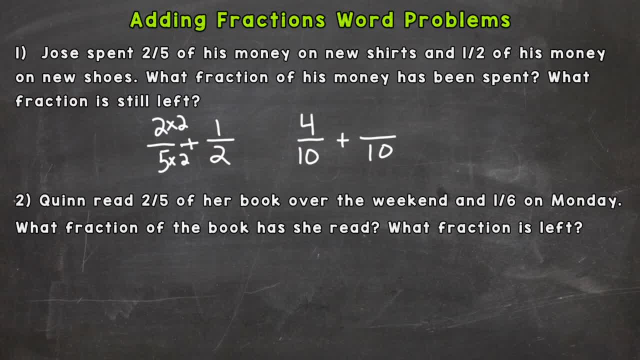 And two times two is four. So two-fifths is four tenths equivalent to four tenths. Now we need to rename one-half. Well, two times five is ten. Let's do that to the top to get our equivalent fraction. One times five is five. Now we're ready to add because we have a common denominator: Four plus five is nine. 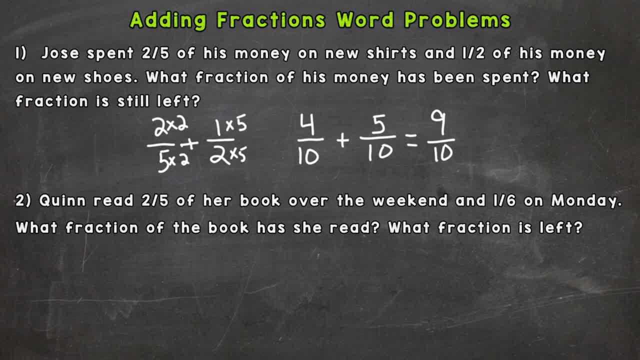 And we keep our denominator of ten the same. So this is how much he spent. He has spent nine-tenths of his money, So nine-tenths has been spent. So now we need to figure out what fraction of his money is left. How do we get to the full? one whole or ten out of ten? So what's left? So if he spent, 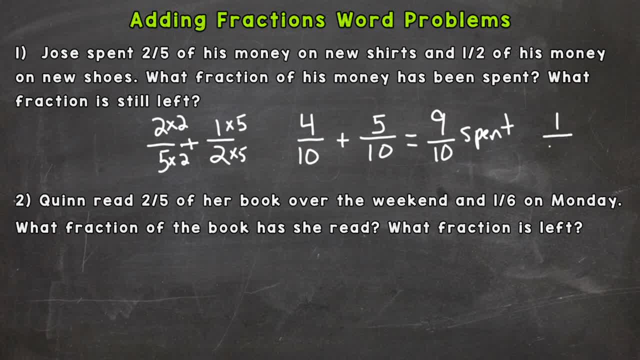 nine-tenths, that means one-tenth is left. That's what we'll get. So now we need to figure out what fraction of his money is left. How do we get to the full? one whole or ten out of ten? So nine-tenths has been. 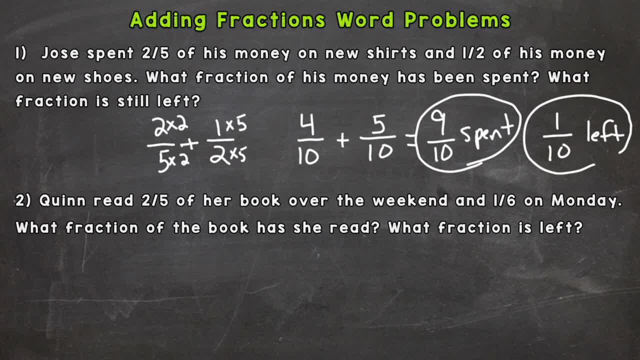 spent, and again one-tenth is left. Let's take a look at number two. Quinn read two-fifths of her book over the weekend and one-sixth on Monday. What fraction of the book has she read? What fraction is left? So again we're. 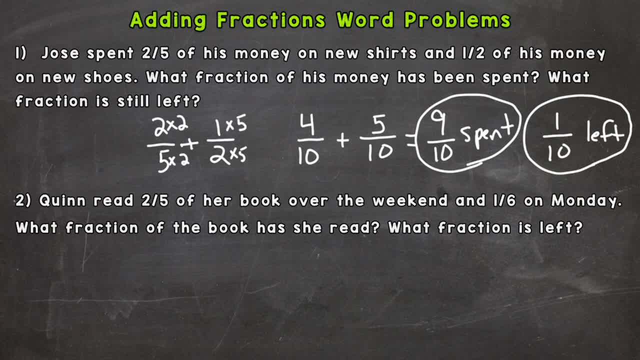 combining two-fifths from the weekend and then one-sixth from Monday, So that's going to be two-fifths plus one-sixth. We do not have a common denominator, so we need to rename with a common denominator. in order to add Five and six, the common denominator is going to be thirty, So let's rename I. 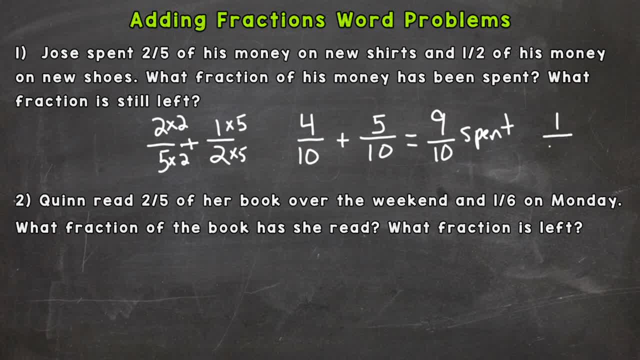 nine-tenths, that means one-tenth is left. That's what we'll get. So now we need to figure out what fraction of his money is left. How do we get to the full? one whole or ten out of ten? So nine-tenths has been. 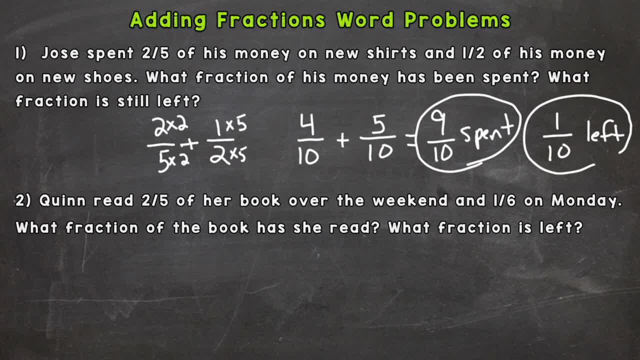 spent, and again one-tenth is left. Let's take a look at number two. Quinn read two-fifths of her book over the weekend and one-sixth on Monday. What fraction of the book has she read? What fraction is left? So again we're. 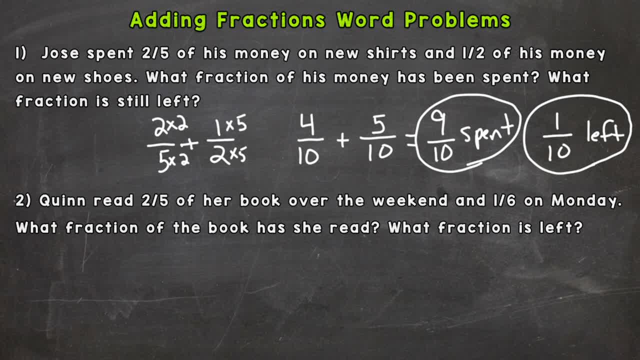 combining two-fifths from the weekend and then one-sixth from Monday, So that's going to be two-fifths plus one-sixth. We do not have a common denominator, so we need to rename with a common denominator. in order to add Five and six, the common denominator is going to be thirty, So let's rename. 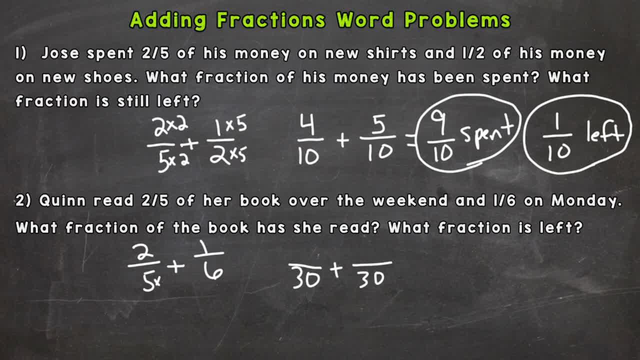 Okay, I know, five times six is thirty, So let's do it to the top. Two times six is twelve. Six times five will give me my denominator of thirty, So I need to do: one times five is five. So here we have twelve plus five is seventeen. Keep our. 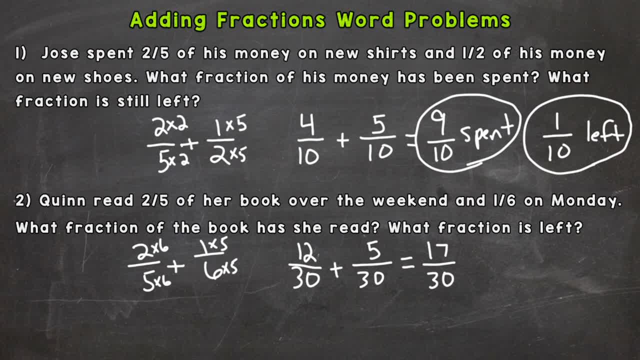 denominator of thirty. So she read: She read a total of seventeen-thirtieths. This is how much she has read. So we need to figure out what fraction is left. How do we get to thirty out of thirty, or one-hundred percent of the book? What's remaining? Well, thirteen-thirtieths would get us to that thirty over thirty, or the one-hundred percent of the book. So we have thirteen-thirtieths left. 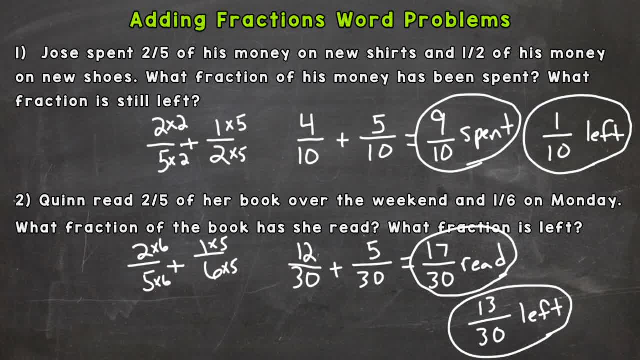 And think about it: Seventeen plus that thirteen gets us to again the thirty out of thirty, which is one whole or one-hundred percent of the book. So there you have it. There's a couple of situations or word problems where we had to add fractions in order to find the solution.